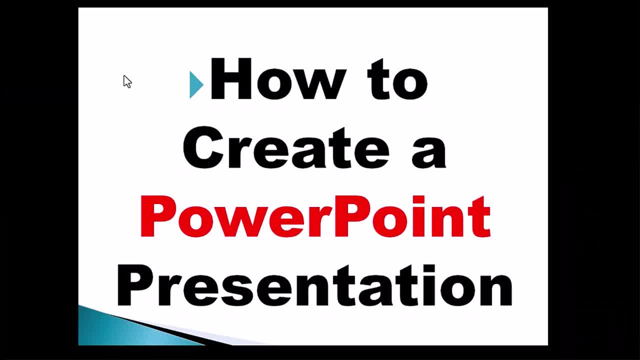 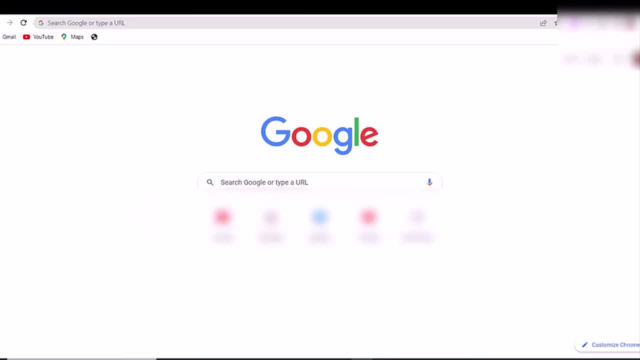 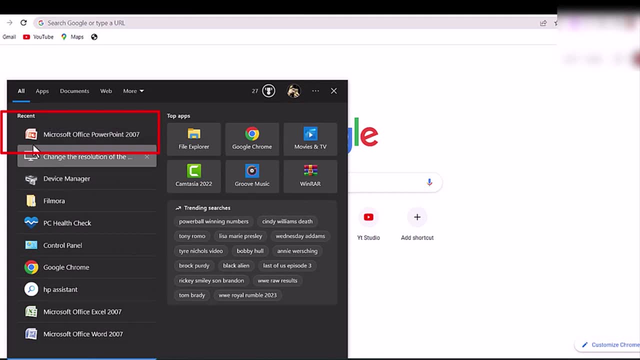 sharing and learning. Today, I will show you how to make a great PowerPoint presentation easily. let's start. The following are steps on how to create a basic PowerPoint presentation. However, certain steps may vary slightly depending upon what version of PowerPoint you are using. 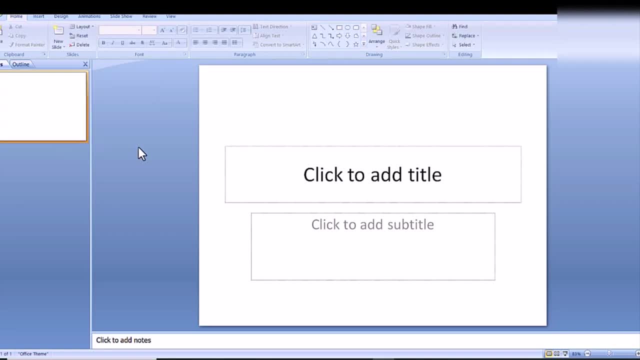 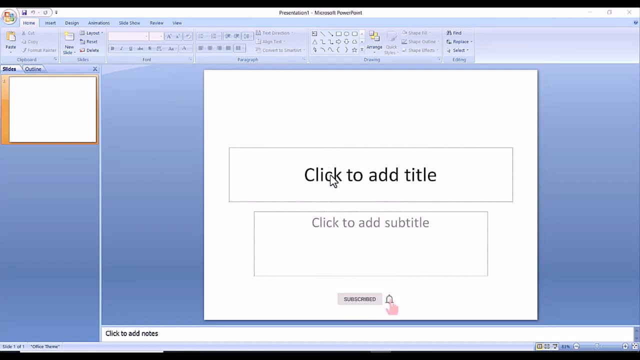 this tutorial is specifically using PowerPoint 2007.. Alright, the step 1 is launch the PowerPoint program. When you launch the PowerPoint program, you may be prompted to pick what kind of document you want to create. Choose to create a blank presentation. if it does not ask you this, a blank presentation will automatically launch. 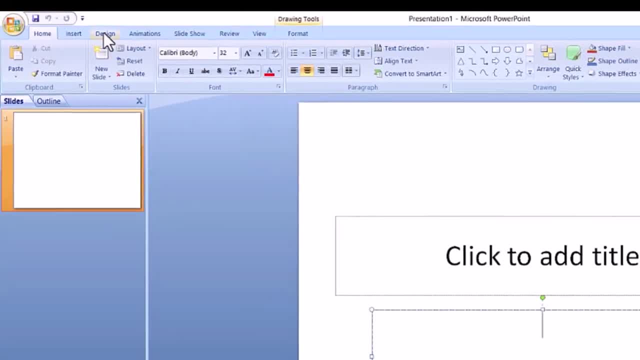 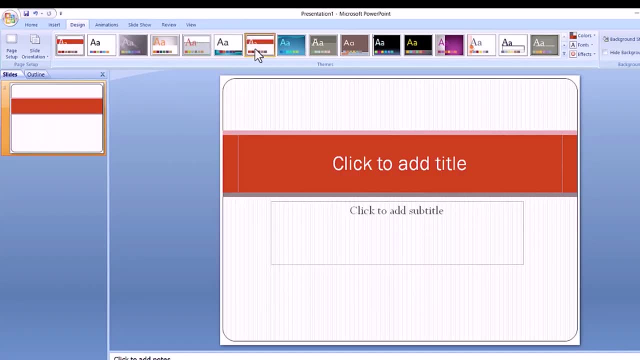 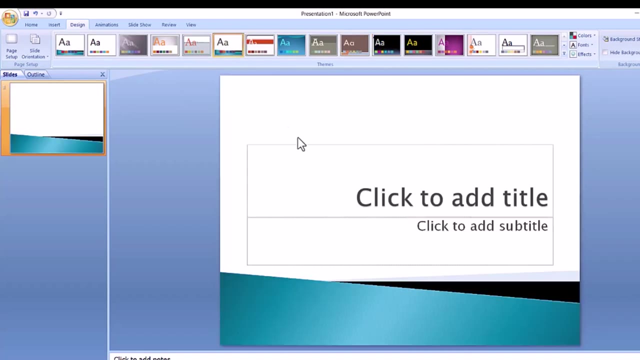 okay, in step two, choosing a design. the next thing you want to do is decide what design you want for the presentation. to do this, go to the design tab at the top of the page, scroll through all the options and decide which one looks best for the presentation you want. this design will be. 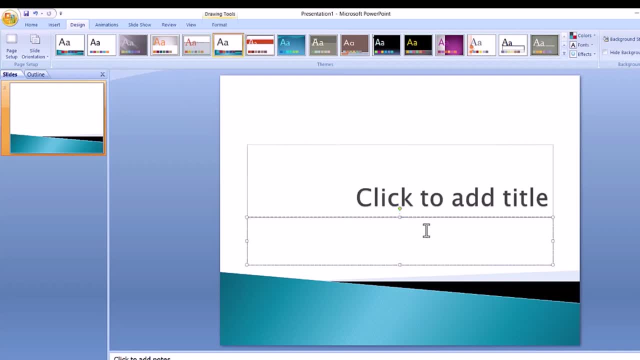 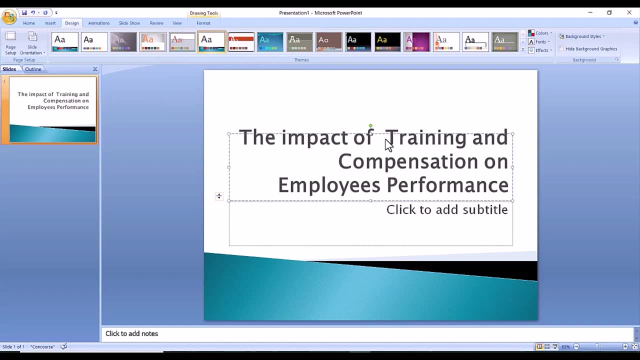 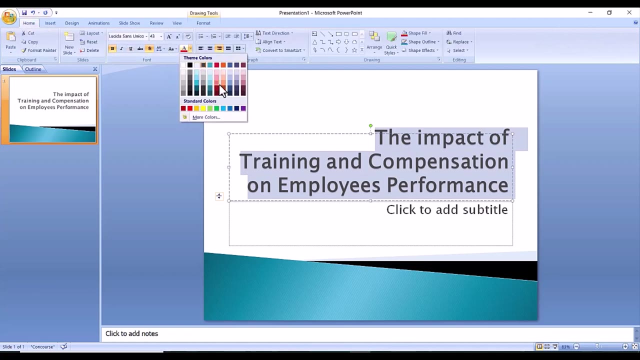 automatically continued throughout the rest of your presentation. step 3: create title page. click the first box that says click to add title and add the title of your presentation. click the bottom box to add your name or any other subtitle that you choose. once you have your text in the 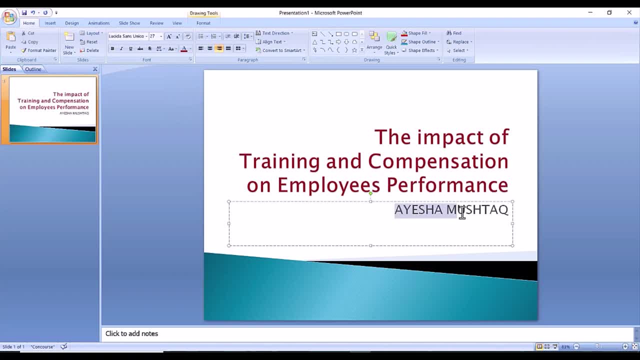 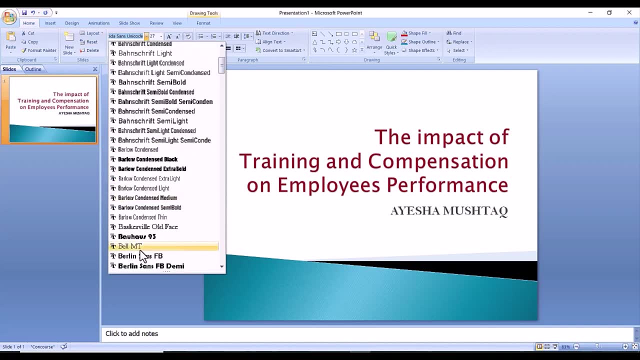 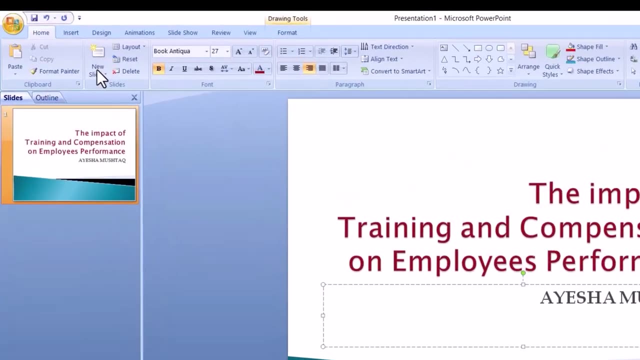 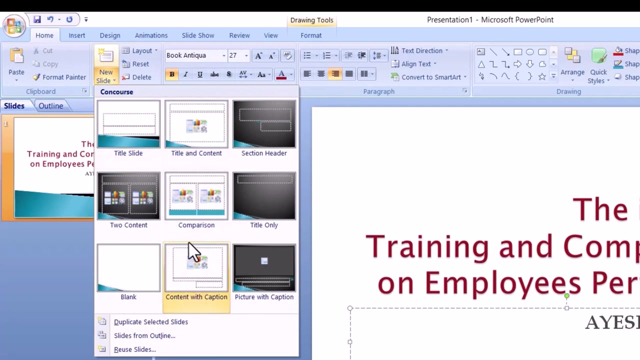 boxes. you can change their font size, color etc. with the toolbar options at the top in step 4, add more slides. chances are you are going to need more than one slide. there are a few ways you can add more slides. notice that there is a separate area to the left. 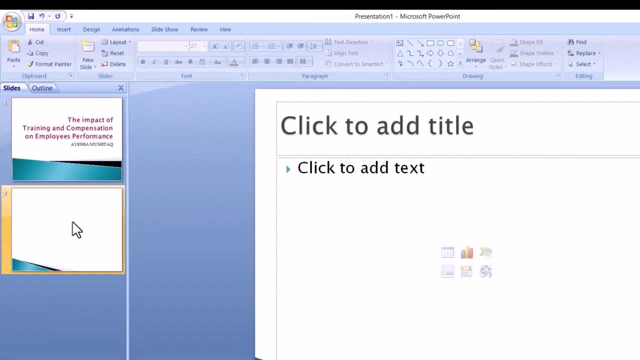 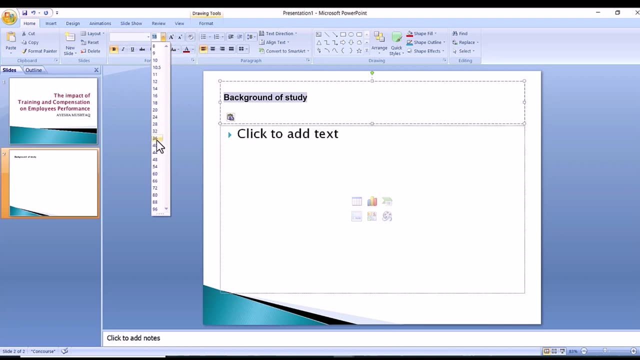 of the screen where your first slide is located. the first way to add a slide is to right click the area under where your first slide is located and select new slide. a new slide will appear. the second way to add another slide it to click new slide in the toolbar above the slides. this. 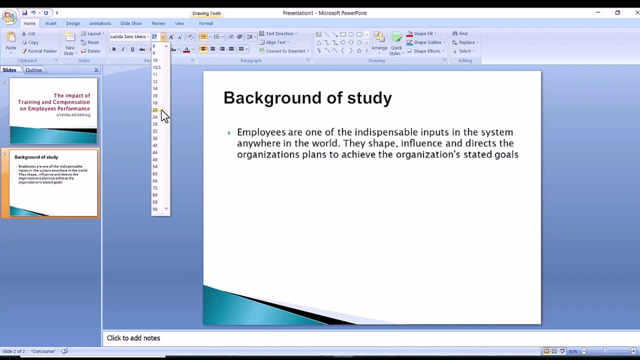 button is divided into two parts. the top will insert a new slide with a default layout. you can also click the bottom half of this button, which will allow you to choose what type of layout you want. you can choose a slide with two text boxes and a title. one text box, only a title. 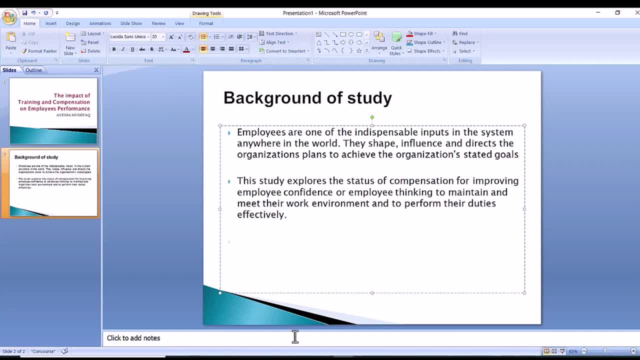 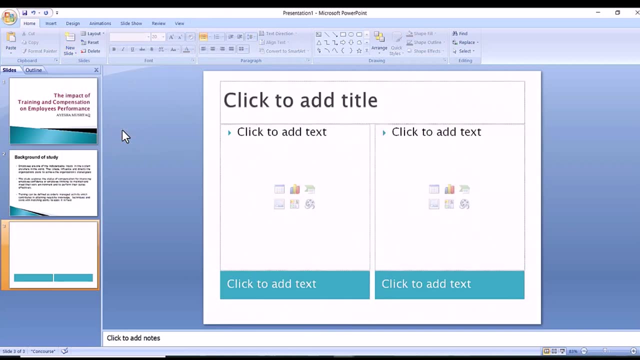 and many other options. you will see your new slide appear to the left under the first, as well become the large slide that you can edit. the design you picked earlier will have carried over to this slide. the design will carry over for the rest of the slides you create, unless you decide to change just one, like described earlier. 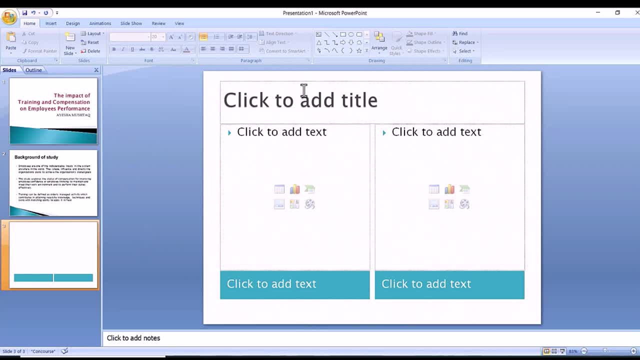 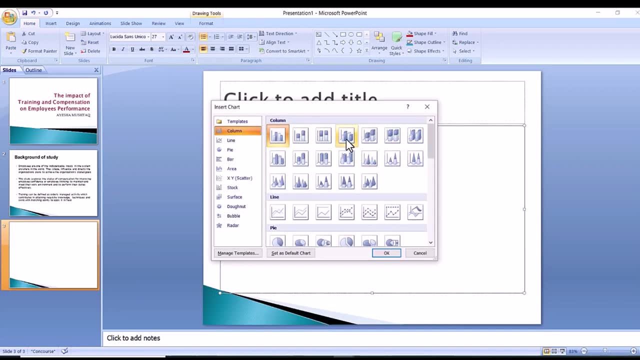 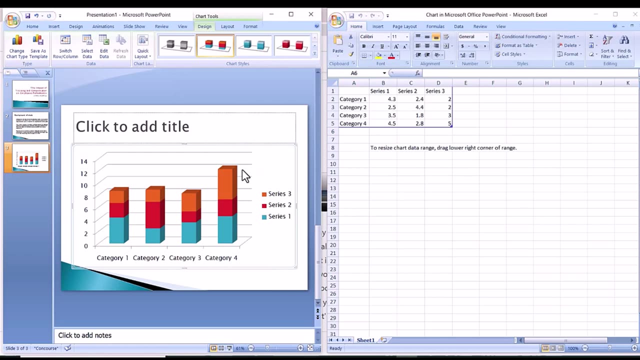 the guideline layout you chose will appear and you can then add in your information. in step 5, add charts, pictures, graphs. if you want to insert a chart, picture, graph or any other graphic, click on the insert tab at the top of the window. here you will see buttons. 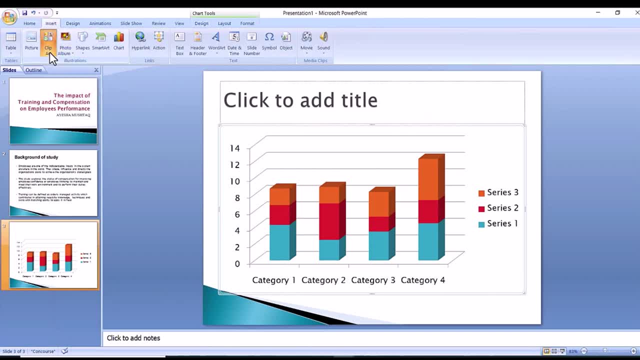 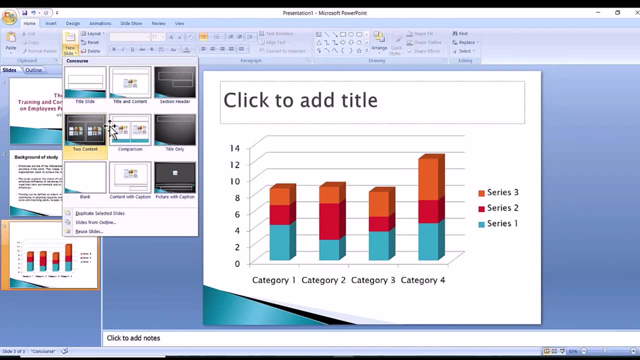 of all the options of what you can insert into your slide. click the designated box and insert what it is you want to have on that slide. a second way you can insert pictures and graphs is when you have an empty text or image box. little pictures of the same options you saw in the 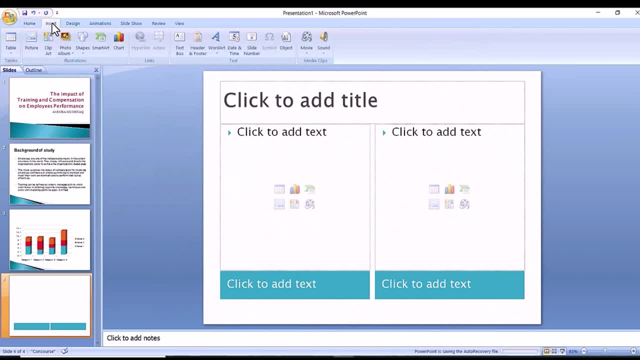 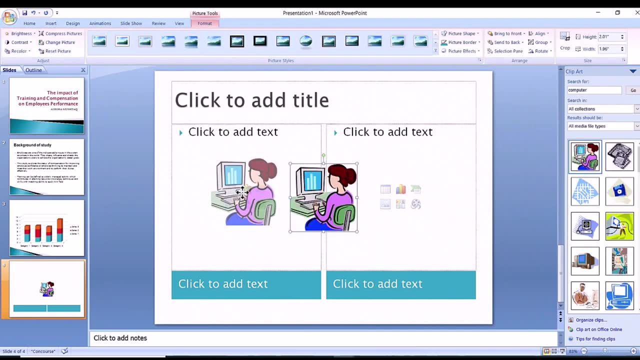 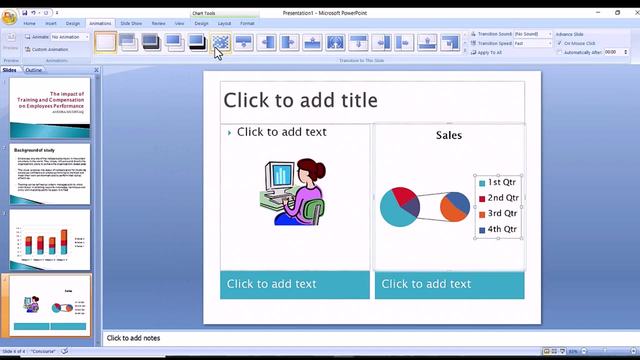 toolbox will show up in the middle of the box and you can click any of these to insert as well once chart or picture. you can add a border or edit it however you want in the format tab okay. next, add transitions. to add transitions in between your slides, click the animations tab at the top. 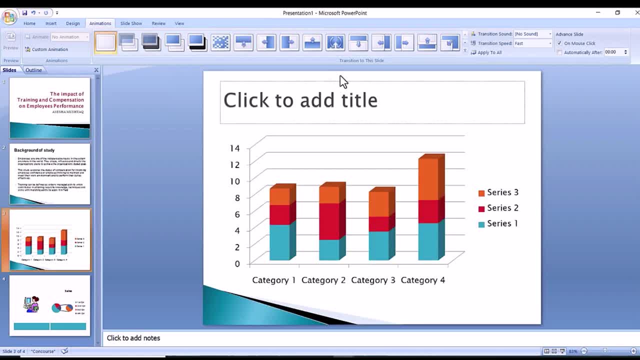 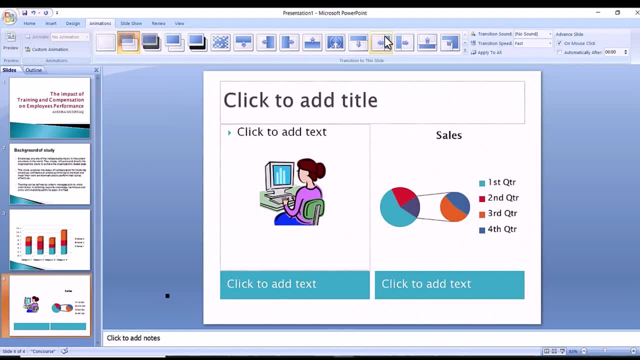 of the page. here you can scroll through all the options of transitions and hover over them to see a preview, select the slide you want the transition applied to and then click the transition you chose. you can do this for every slide, selecting the same transition when submission is applied to slide. and watch out the chart for transitions to add. 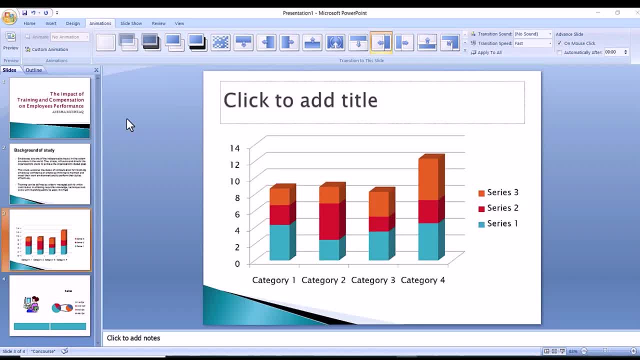 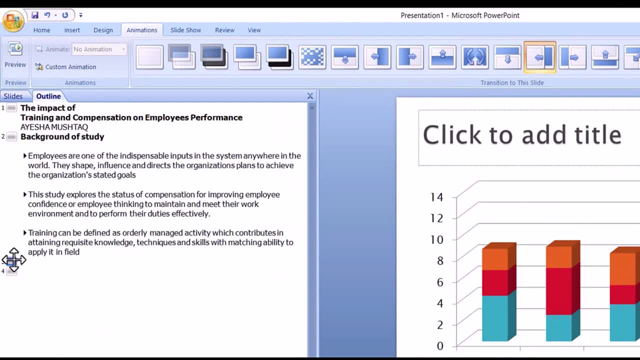 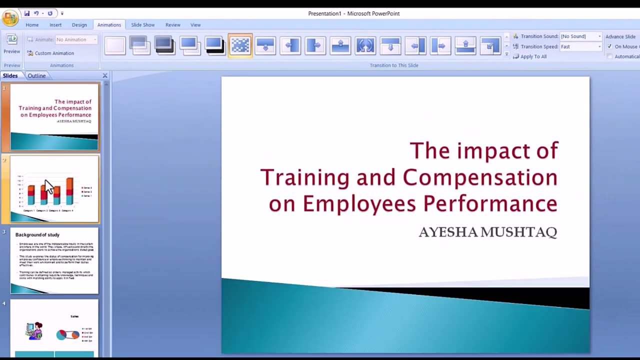 same or different transitions. Next, changing the order. once you have all your slides made, you can change the order of the slides. to do this, click and drag the slides from where they are to where you want them in the order. another possibility which is particularly useful if you presentation. 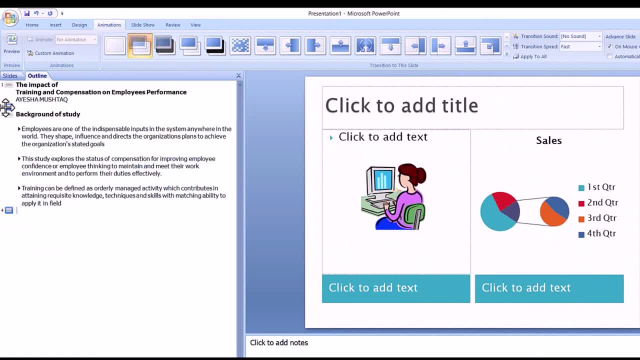 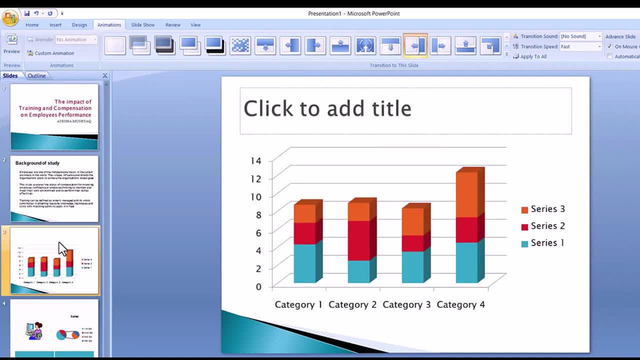 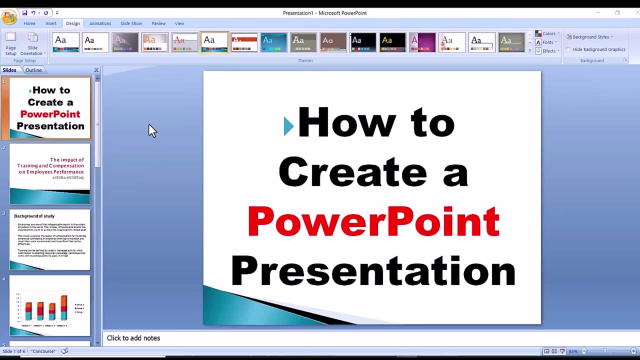 is longer is to click the outline button. You can find this small button above the left area where all your slides are located, smaller, directly to the right of the slides button. here you will see a list of all your slides and you can click and drag your slides to where you want them.